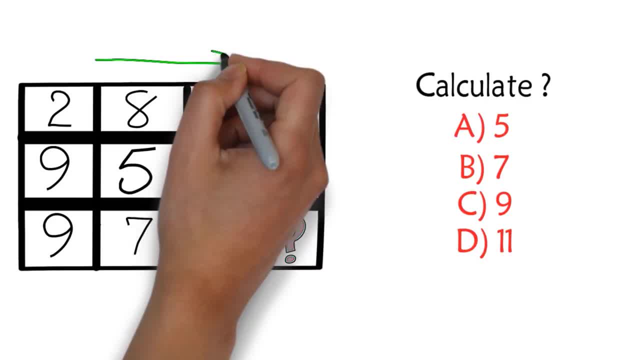 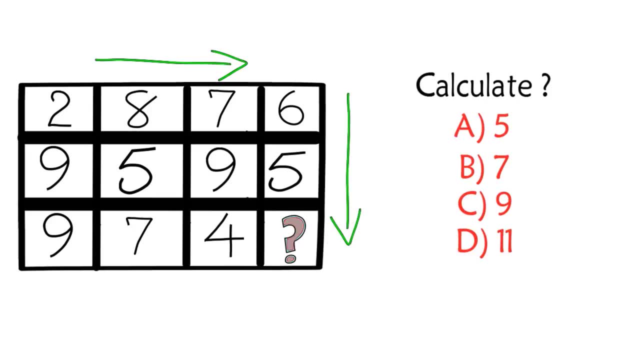 The key to solve this problem is to determine the pattern, And the pattern either can be in the rows or in columns. In this particular case, let's check the columns first, And then what you see is that each column adds up to the value of 20.. For example, 2 plus 9 plus 9 is 20.. 8 plus 5 plus. 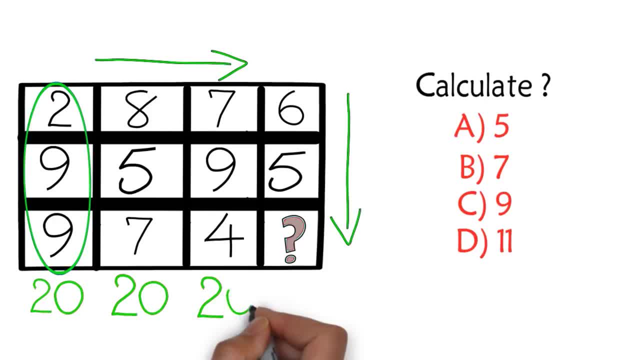 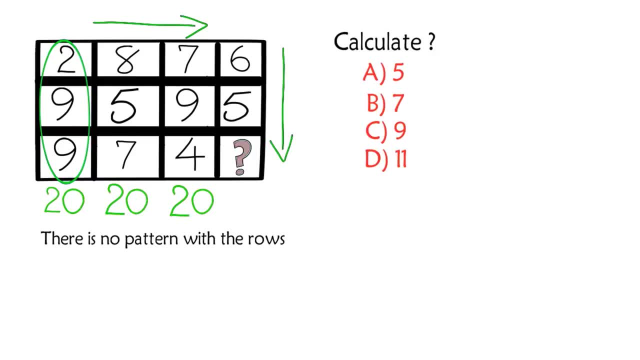 7 is 20.. 7 plus 9 plus 4 is 20 as well. We also want to check if there is a pattern with the rows. And there is no pattern, Because the first row adds up to 23.. 2 plus 8 plus 7 plus 6 equals 23.. 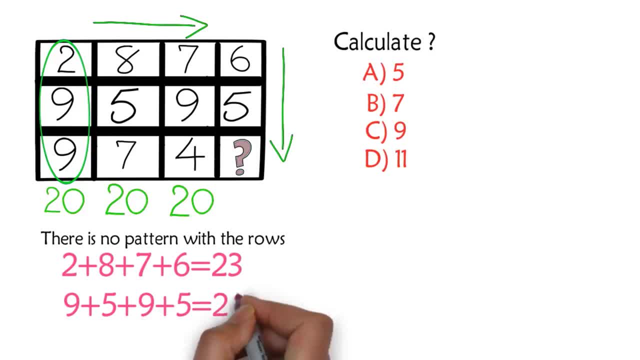 And the second row adds up to 28.. 9 plus 5 plus 9 plus 5 equals 28.. So there is no pattern. Based on this information, you can calculate the missing value in the fourth column: 6 plus 5 plus question mark equals 20.. So the answer is C 9.. This is the missing value. 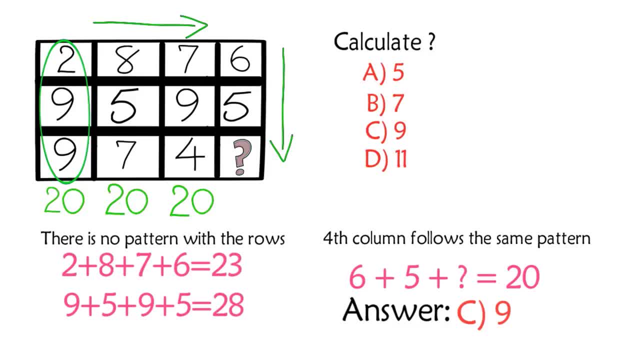 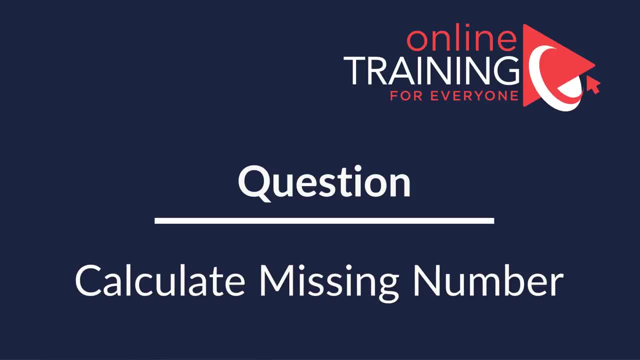 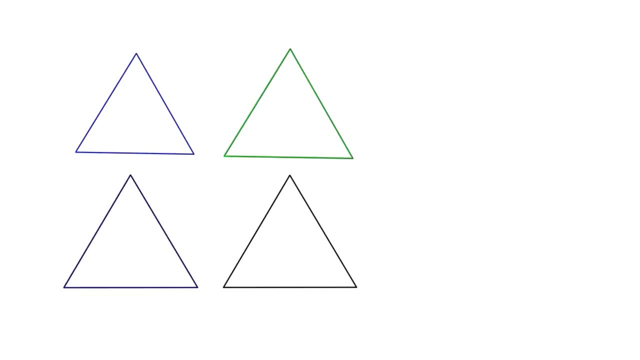 Hopefully you figured it out and now know how to answer similar problems on the test. Here is another puzzling question you might find difficult to solve. You are presented with four triangles. Each triangle has a number in the corner And you need to calculate one of the missing numbers in the upper corner of the black triangle. 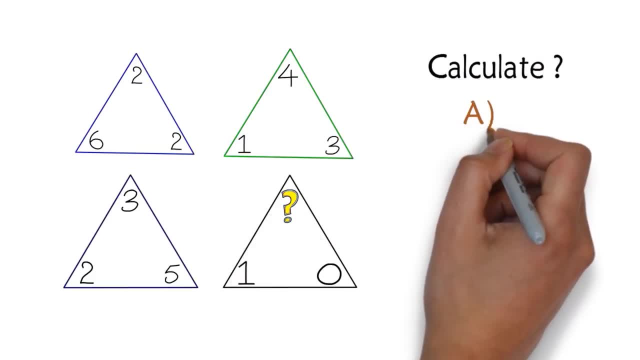 You have four different choices. You have choice A, 1. You have choice B: 2. You have choice C: 3. And you have choice D, 4.. Can you determine the answer? Let's continue to see how we can solve this challenge together. 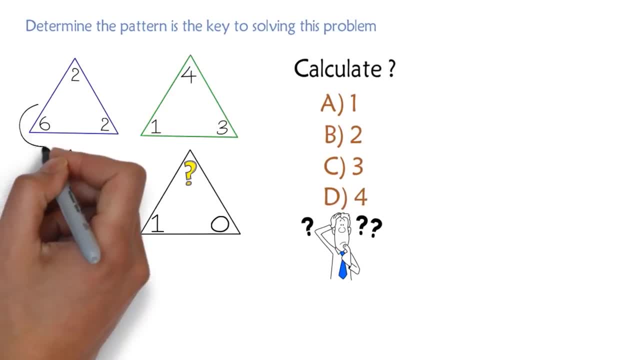 Determining the pattern is the key to solving this challenge. For example, if you add up the numbers in the lower left corners, 6 plus 1 plus 1 plus 2 in all triangles, you will get to the sum of 10.. 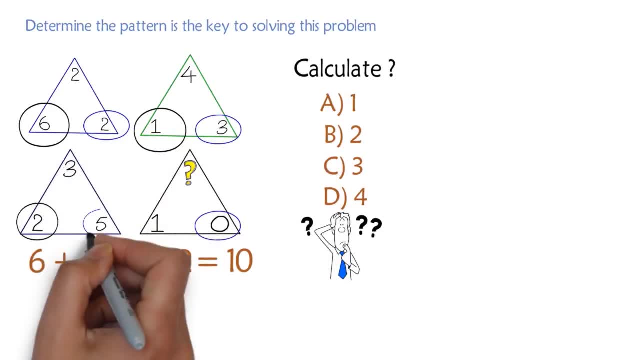 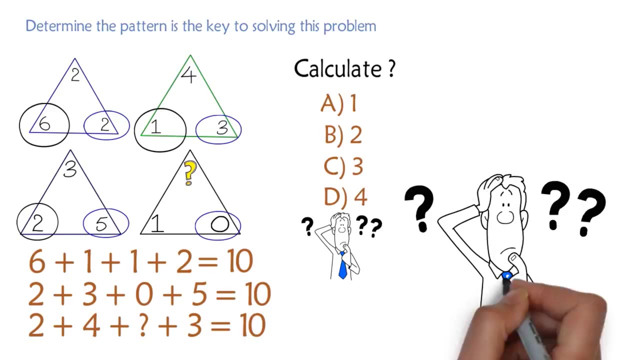 Same thing happens when you add up the numbers in the bottom right corners of the same triangles: 2 plus 3 plus 0 plus 5 also equals 10.. So same logic can be applied to the upper right corners of the triangles. As you can see, triangles are colored to confuse you. 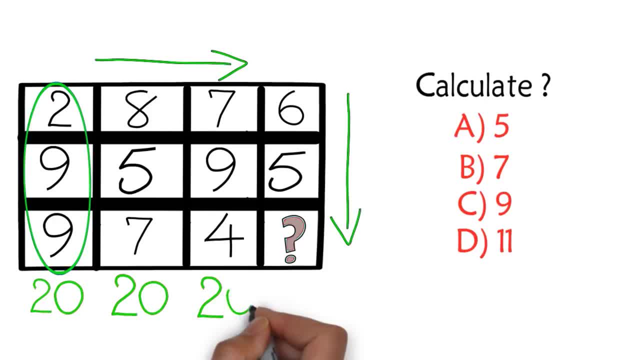 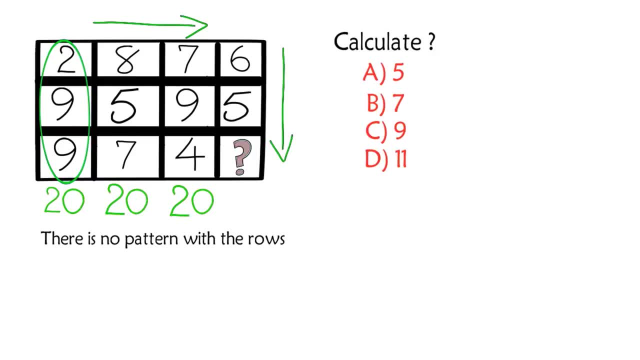 7 is 20.. 7 plus 9 plus 4 is 20 as well. We also want to check if there is a pattern with the rows. And there is no pattern, Because the first row adds up to 23.. 2 plus 8 plus 7 plus 6 equals 23.. 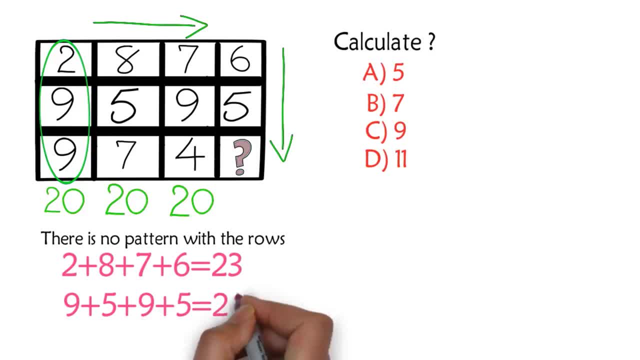 And the second row adds up to 28.. 9 plus 5 plus 9 plus 5 equals 28.. So there is no pattern. Based on this information, you can calculate the missing value in the fourth column: 6 plus 5 plus question mark equals 20.. So the answer is C 9.. This is the missing value. 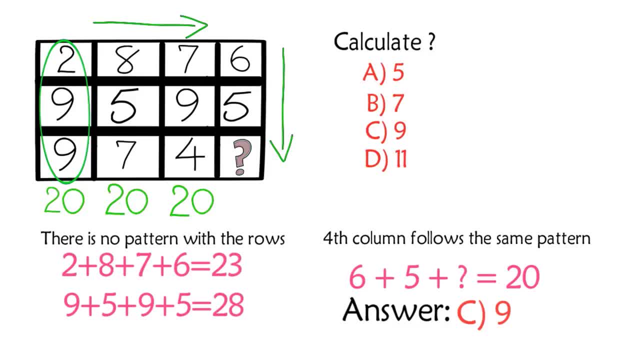 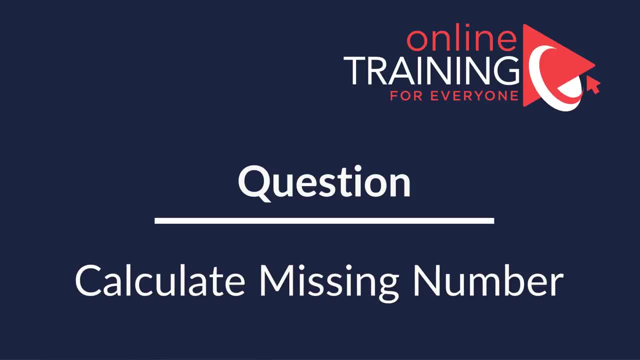 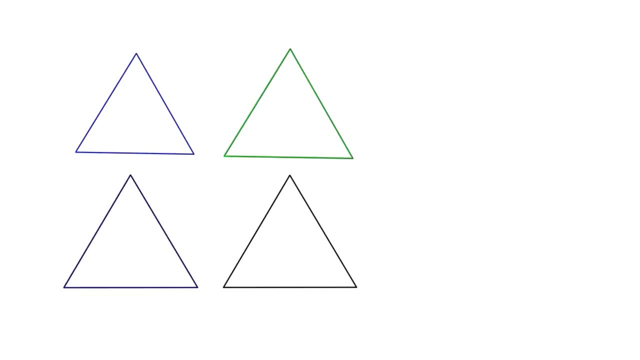 Hopefully you figured it out and now know how to answer similar problems on the test. Here is another puzzling question you might find difficult to solve. You are presented with four triangles. Each triangle has a number in the corner And you need to calculate one of the missing numbers in the upper corner of the black triangle. 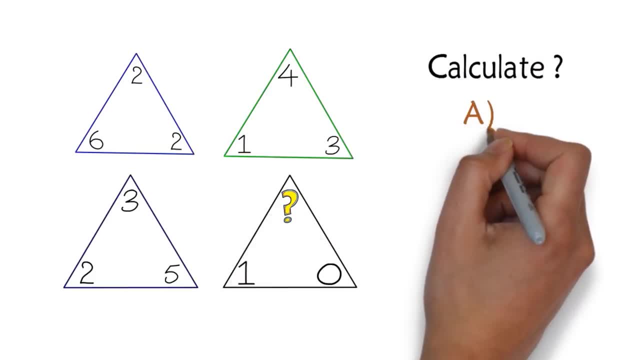 You have four different choices. You have choice A, 1. You have choice B: 2. You have choice C: 3. And you have choice D, 4.. Can you determine the answer? Let's continue to see how we can solve this challenge together. 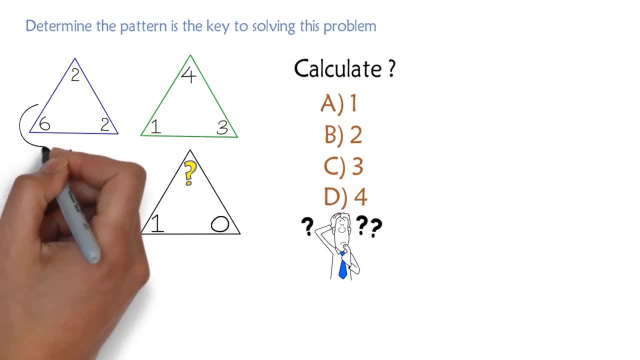 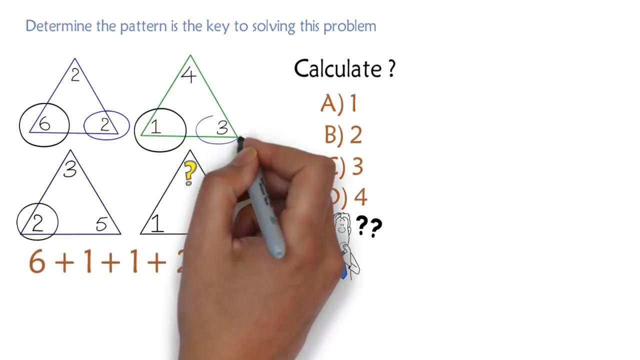 Determining the pattern is the key to solving this challenge. For example, if you add up the numbers in the lower left corners, 6 plus 1 plus 1 plus 2, in all triangles, you will get to the sum of 10.. Same thing happens when you add up the numbers in the 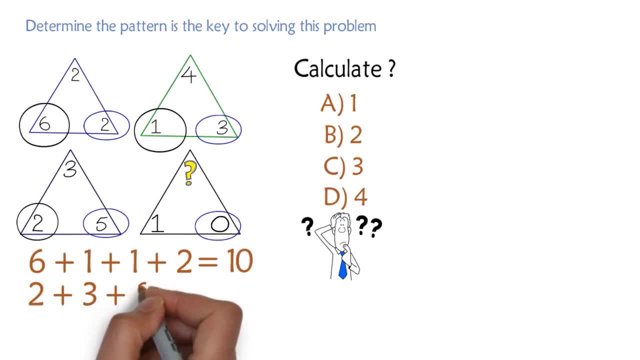 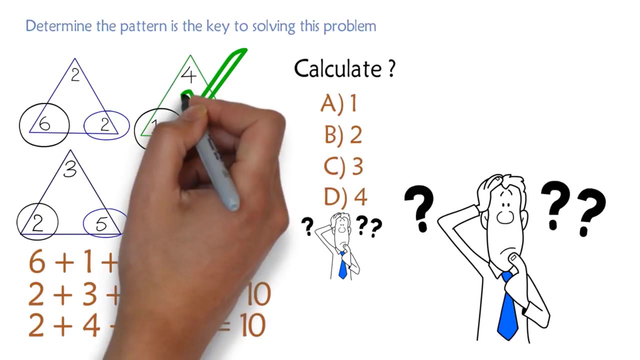 bottom right corners of the same triangles. 2 plus 3 plus 0 plus 5 also equals 10.. So same logic can be applied to the upper right corners of the triangles. As you can see, triangles are colored to confuse you, So you're only concentrated on the numbers inside of each triangles. But you're 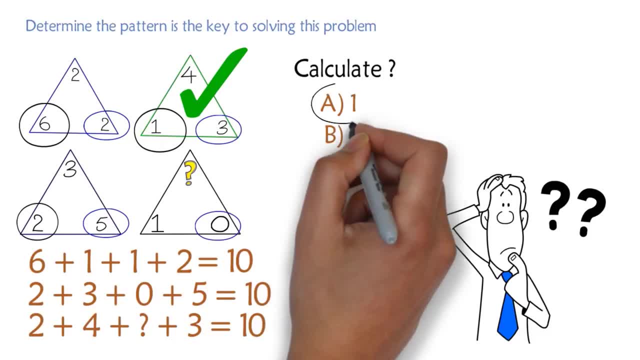 not looking across multiple triangles. The correct answer to this problem is choice A 1. Because this is the math of getting into 10 with the missing numbers. So you have choice A 1. And you can get straight to the answer. Up to 10 per triangle is also the number that you need, knowing that. 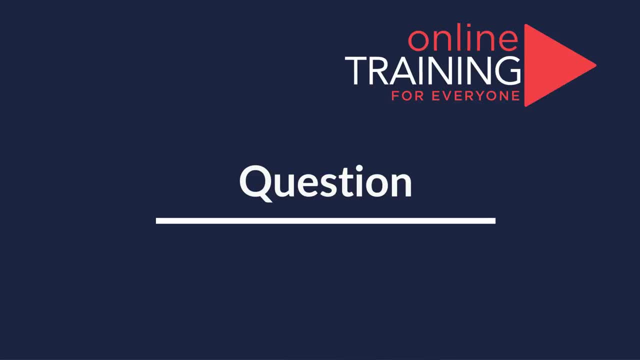 if we add up each of the KongMusic Okkai triangles, you won't need them. You don't need to slightly ада, Stefan, but you can add up to 10. You can figure it out only if you get a better answer. 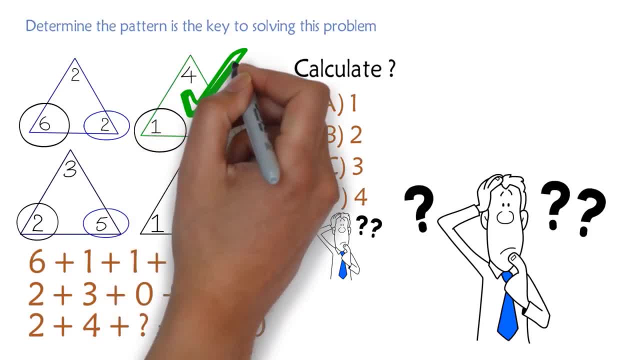 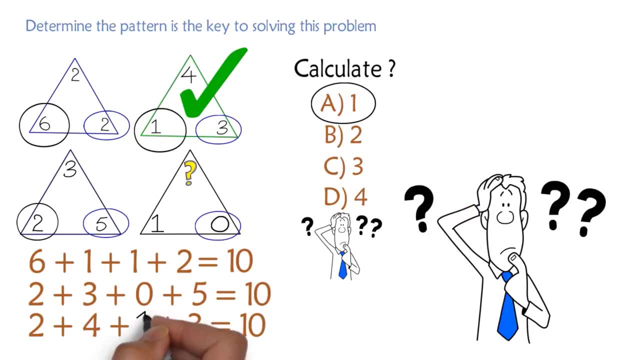 So you are only concentrated on the numbers inside of each triangles, but you are not looking across multiple triangles. The correct answer to this problem is choice A, 1, because this is the math of getting into 10 with the missing number. Hopefully you've nailed this question and now know how to answer similar problems on the test. 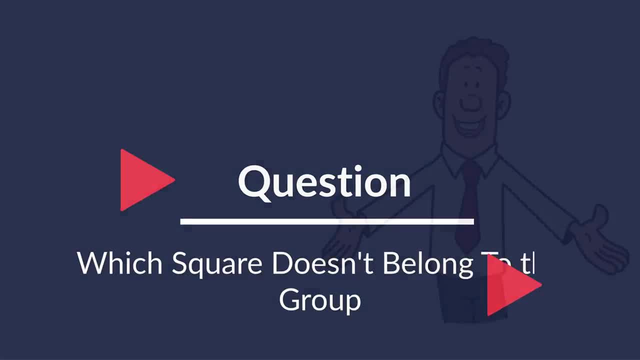 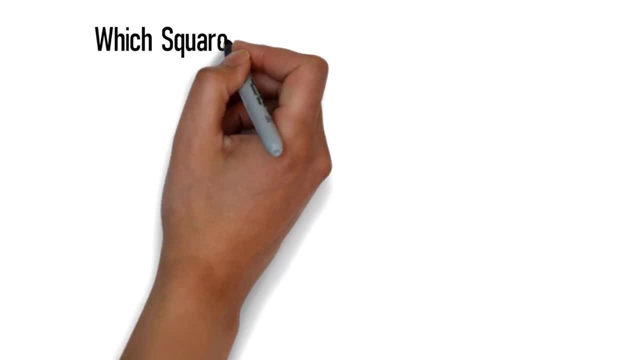 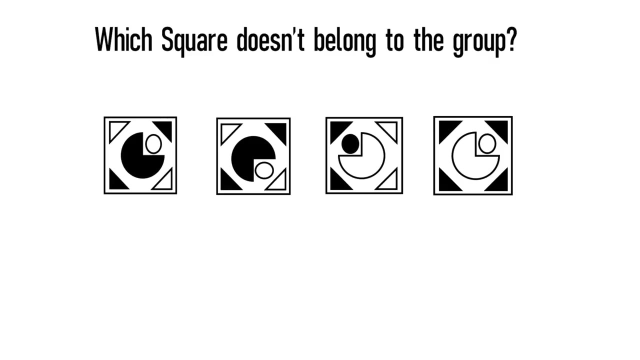 I am excited to take advantage of the opportunity and share with you how to solve these types of problems on the test. Typically, when you get a problem, you need to determine which object does not belong to the group. In this particular case, you need to determine which square doesn't belong to the group. 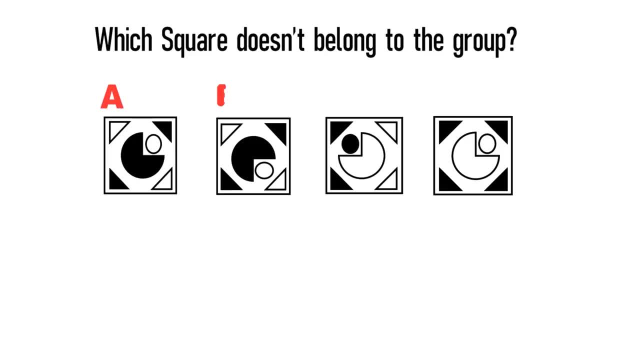 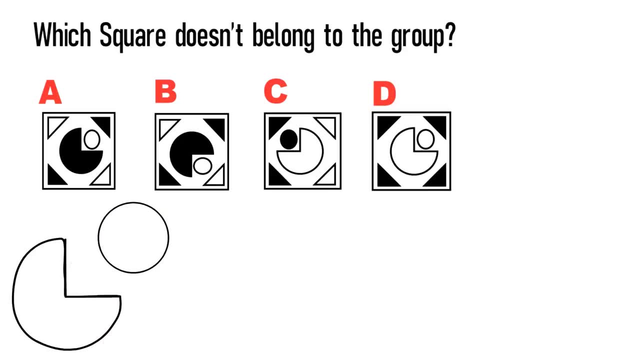 You are presented with four different squares: Choices A, B, C and D. Each square contains two circles inside. In the large circle, quarter of each circle is missing and instead replaced with the small circle. All squares also have triangles in the corner. 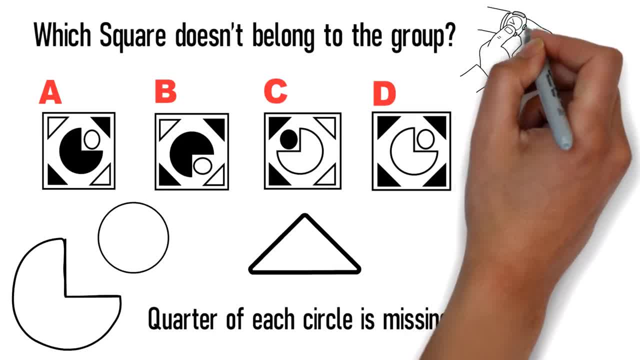 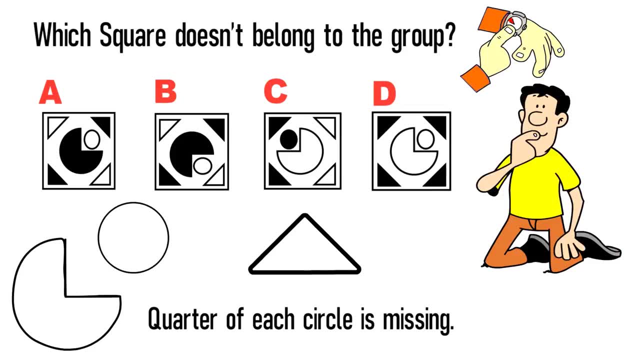 Give yourself 5 to 10 seconds to see if you can come up with the answer. Do you see the answer? Let's continue to see how we can solve this challenge and get to the correct solution together. The key to solving this challenge is to detect the pattern. 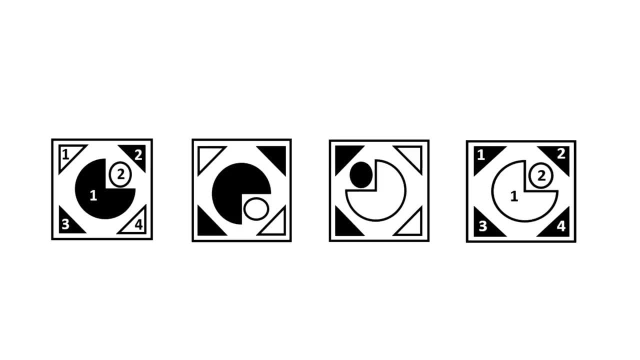 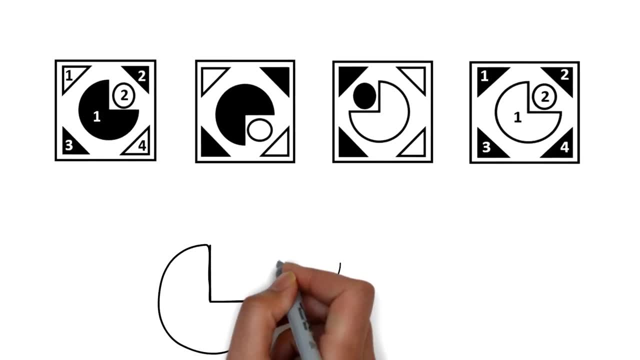 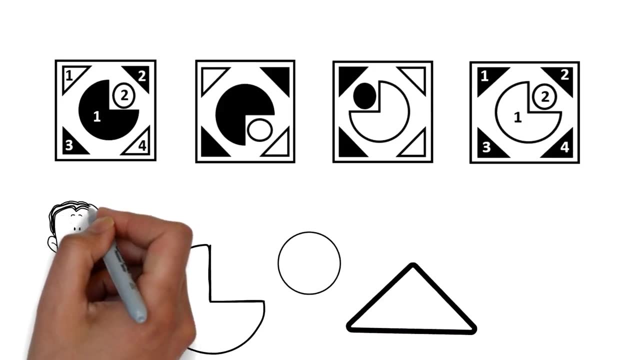 This is the skill that you need to develop to be successful in the test. Because there are two shapes here present in this question: triangles and circles. you should try to detect the pattern among triangles and then among circles. In this particular question, there is only one pattern pattern of the triangles. 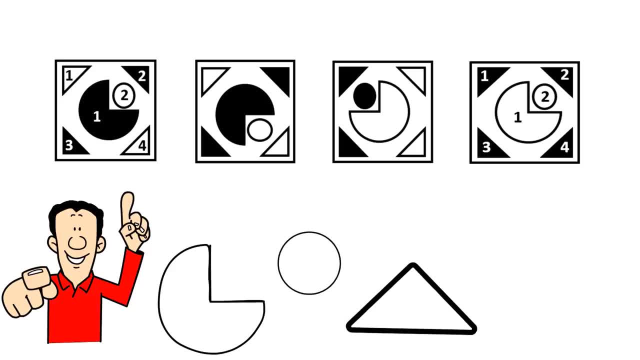 But there are some sophisticated questions on the test which might include patterns for both shapes. In this particular case, the pattern is that the square should contain the equal number of black and white triangles in the corners Triangles in the square A, positioned diagonally across each other. 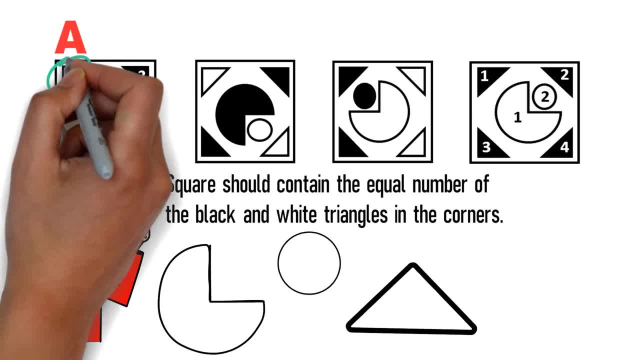 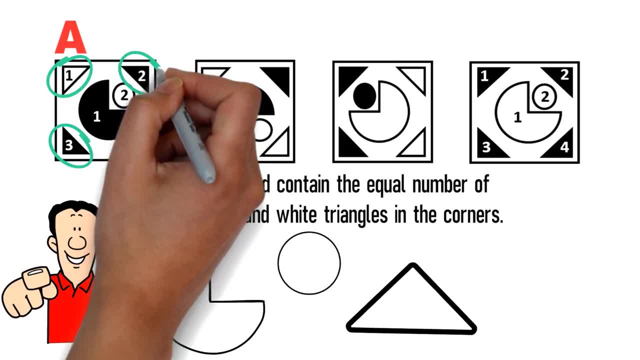 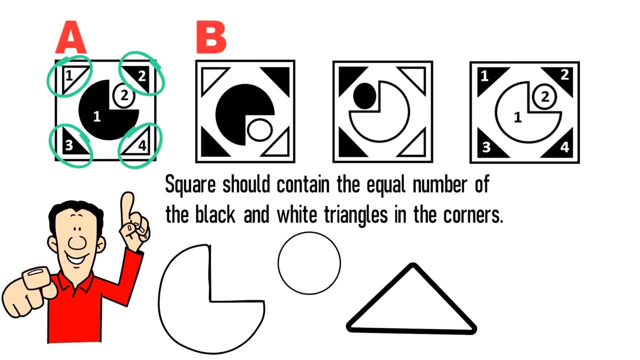 White triangles are located in the upper left corner and in the bottom right corner, And black triangles are located in the bottom left corner and in the upper right corner. You can see that the same pattern exists in the shape B: two white triangles and then two black triangles. 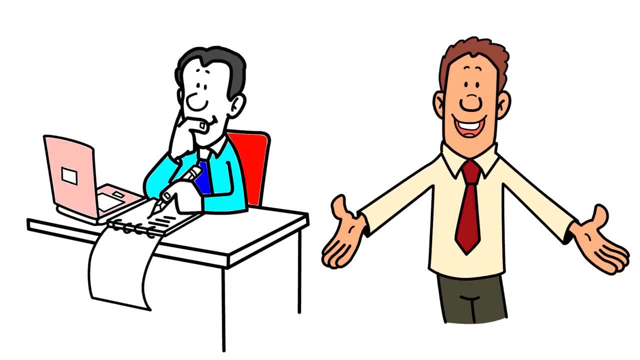 Finally, if you want to closet, bring theindet together on top of a crossed circle, a parallel triangle can pop up on top of the triangle or simply put it into the reverse angle next to it. To how we can solve such English assignment challenge, you can use an electronicRaеч. 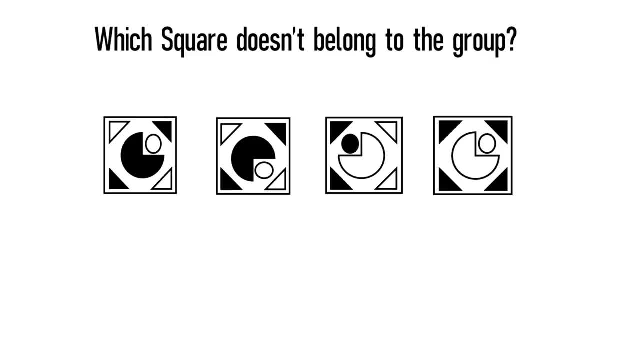 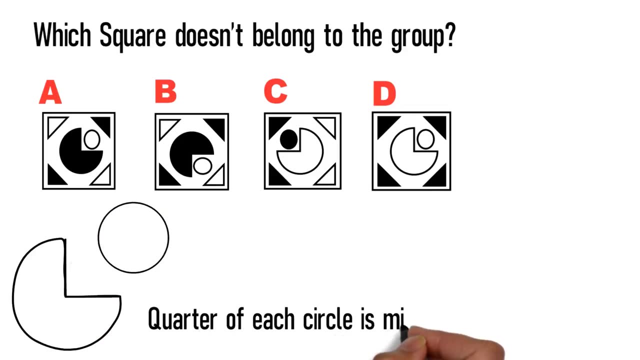 applied in your favorite room and put it on our prof whale project. We justroull from here to our table. Choices A, B, C and D: Each square contains two circles. inside. In the large circle, quarter of each circle is missing and instead replaced with the small. 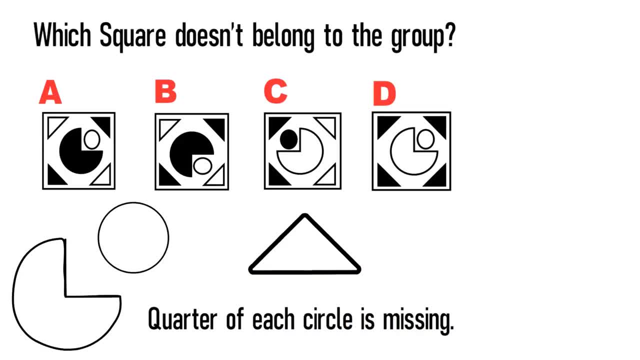 circle. All squares also have triangles in the corner. Give yourself 5 to 10 seconds to see if you can come up with the answer. Do you see the answer? Let's continue to see how we can solve this challenge and get to the correct solution. 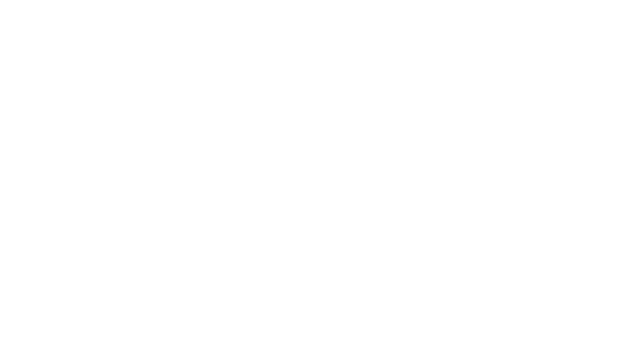 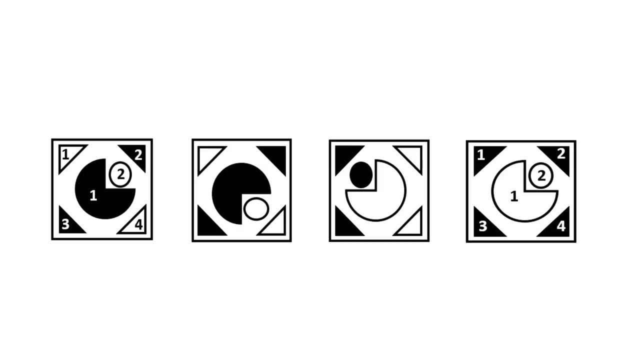 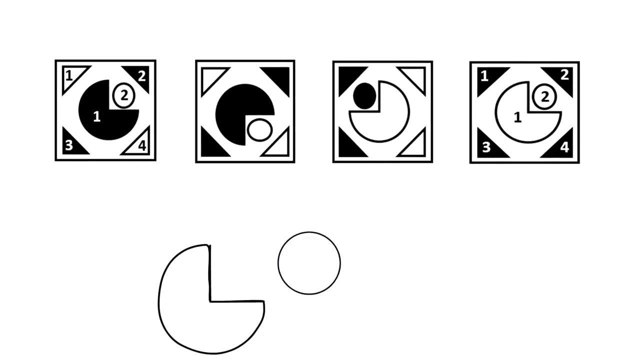 together. The key to solving this challenge is to detect the pattern. This is the skill that you need to develop to be successful in the test, Because there are two shapes here present in this question: triangles and circles. you should try to detect the pattern among triangles and then among circles. 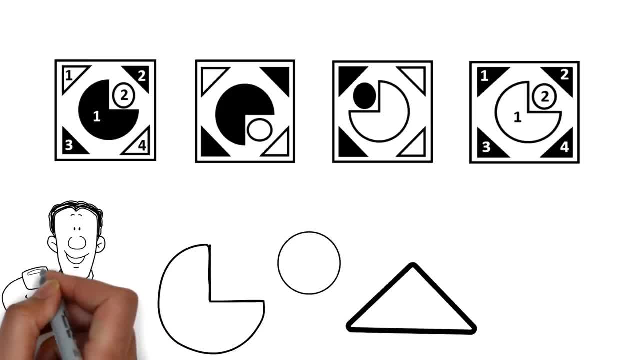 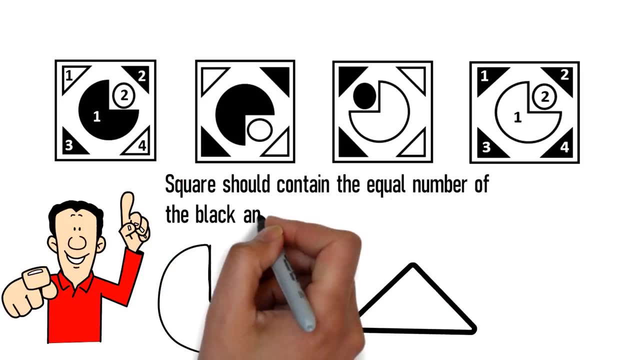 In this particular question there is only one pattern pattern of the triangles, But there are some sophisticated questions on the test which might include patterns for both shapes. In this particular case, the pattern is that the square should contain the equal number of black and white triangles in the corners. 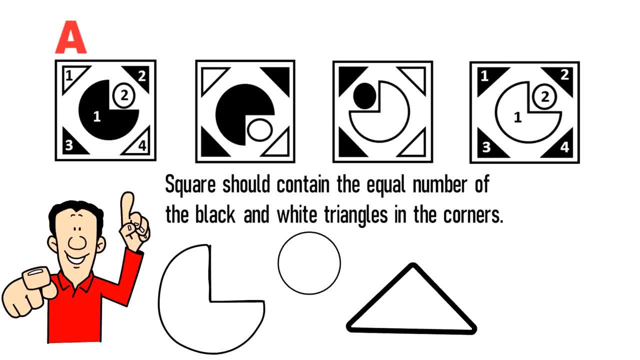 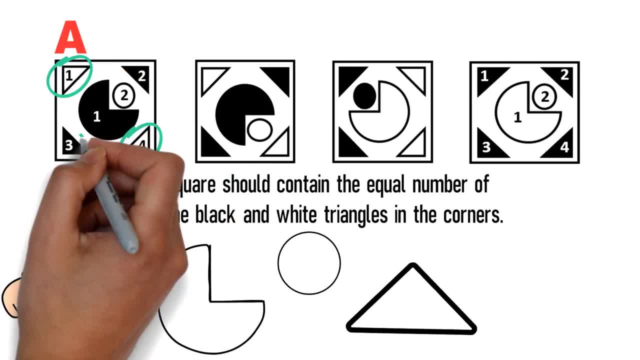 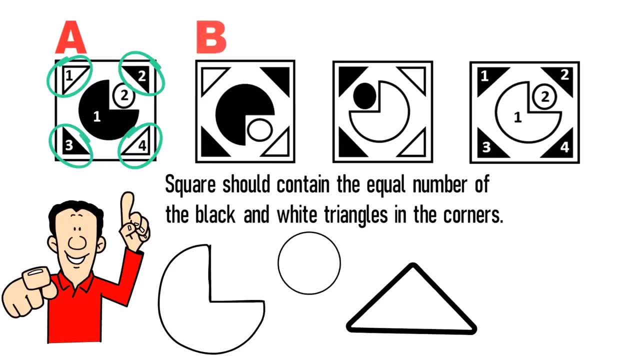 Triangles in the square A, positioned diagonally across each other. white triangles are located in the upper left corner and in the bottom right corner, and black triangles are located the bottom left corner and in the upper right corner. you can see that the same pattern exists. 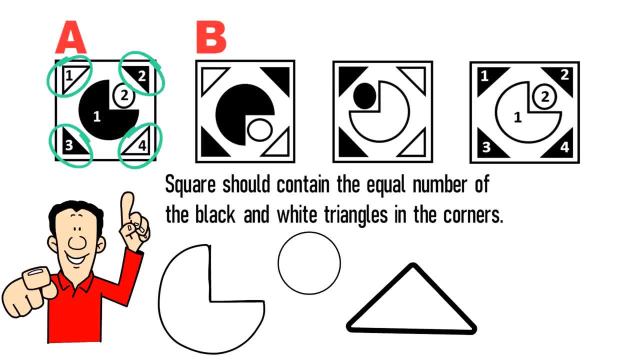 in the shape b two white triangles and then two black triangles, and in the shape c two black triangles on the left and two white triangles on the right. but if we look at the choice d you see that there are four black triangles in the corners. circles in this picture do not have 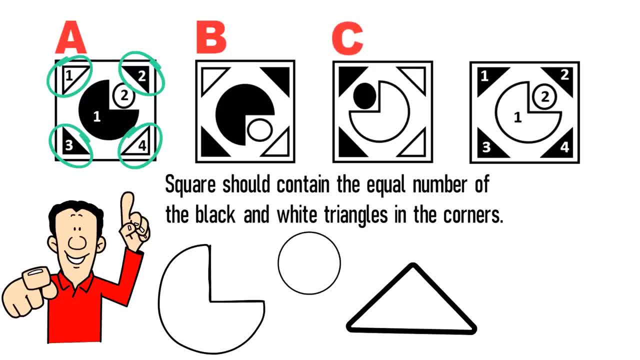 and in the shape C, two black triangles on the left and two white triangles on the right. But if we look at the choice D, you see that there are four black triangles in the corners. Circles in this picture do not have a pattern and their primary goal is to confuse you. 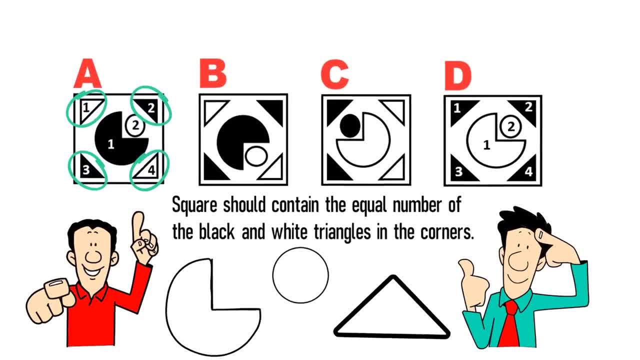 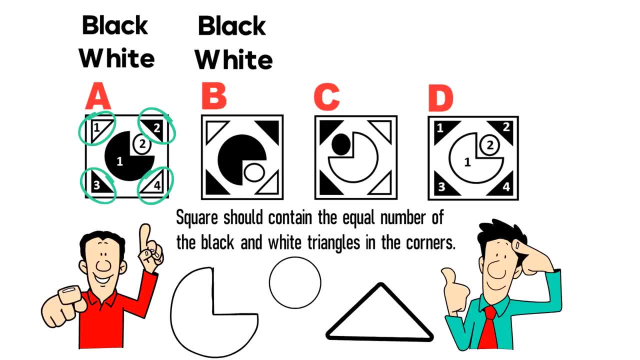 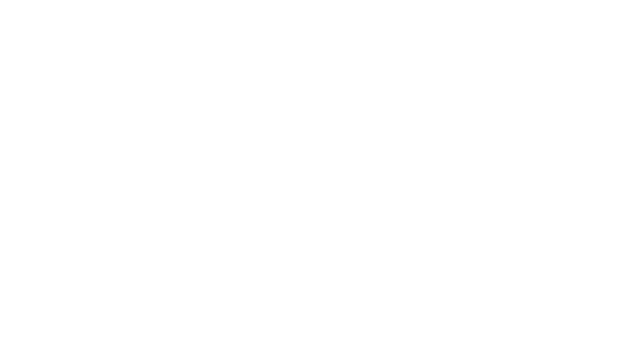 If you look at the circles closely, you see that the large small circle pattern does not exist. We have black-white shape B black-white, shape C- white-black and then shape D- white-white. Based on this information about the circles, we should ignore them. 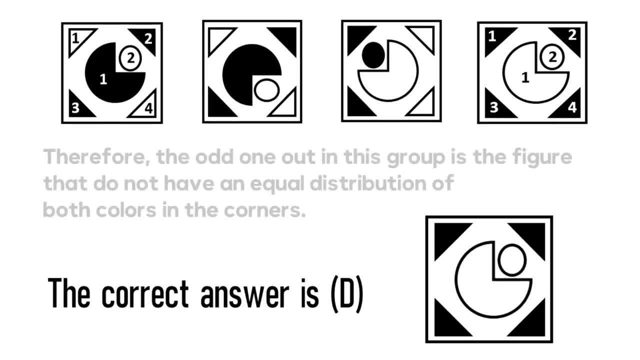 and focus on the triangles inside the squares. This is why the odd shape, the shape that doesn't belong to the group, is the one that does not have equal distributions of all colors in the corners. So the correct answer here is choice D. 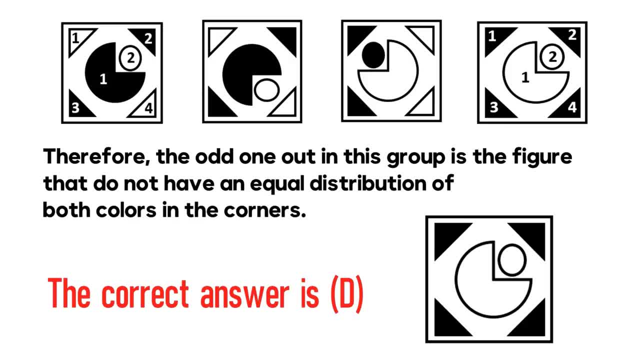 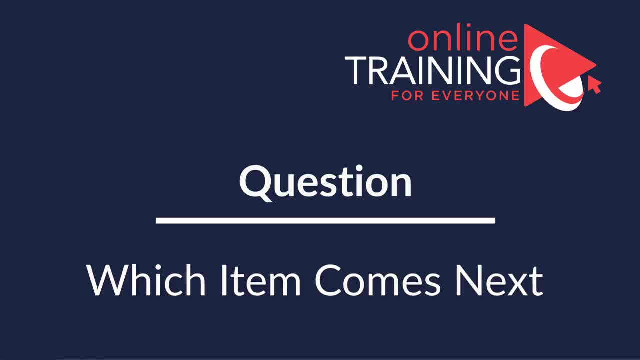 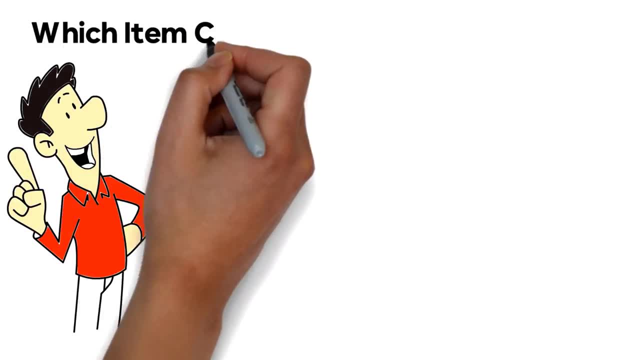 Hopefully you've nailed this question and now know how to answer similar problems on the test. Very frequently on the test you might be asked to detect the pattern. In this question we are being asked which item comes next in the sequence and we are presented with the sequence of items. 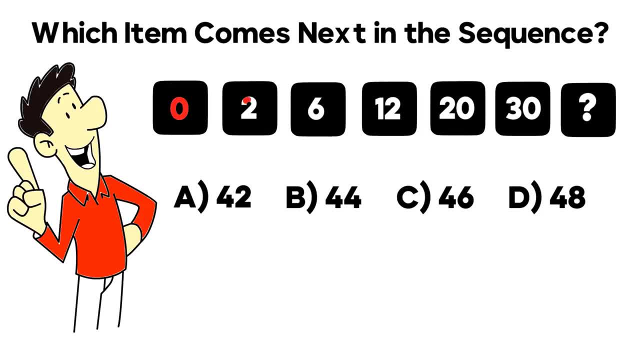 Six items in the sequence are visible: 0, 2, 6, 12, 20 and 30.. And the next item is missing and you are being asked to select one of the four following choices: Choice A- 42.. Choice B: 44.. 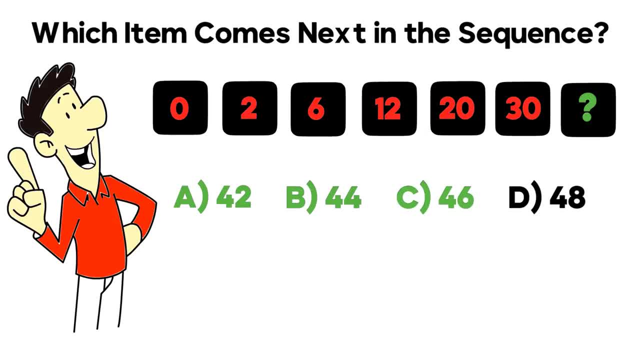 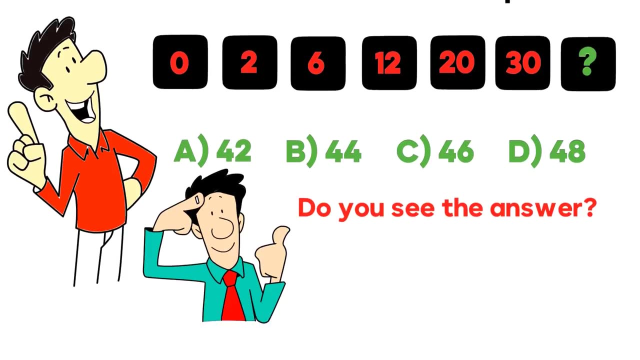 Choice C: 46. And choice D: 48.. Do you see the answer? It may or may not be obvious, depending upon your skills of detecting the pattern, Like it or not. we are going to continue and I'll share with you the answer. 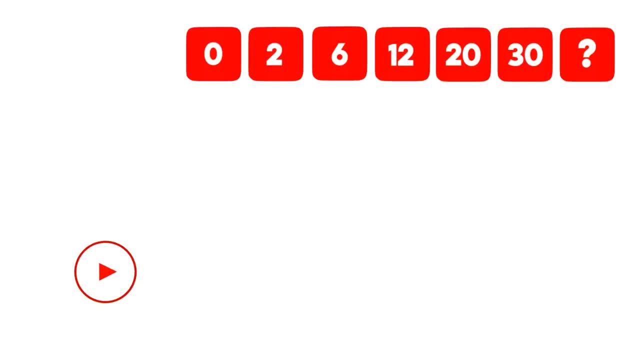 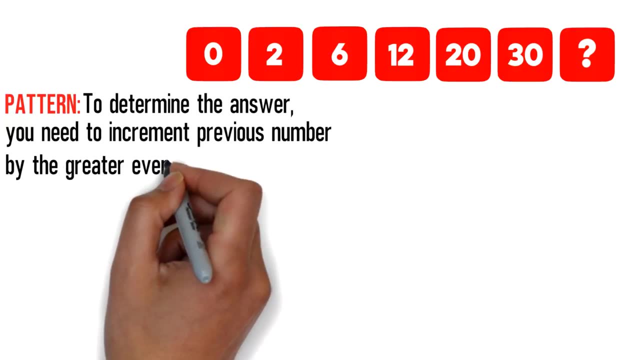 As with any type of question, the key is to determine the pattern, To determine the answer. in this particular case, you need to increment the previous number by the greater even digit. in the sequence, You can even come up with the formula And, in our case, the formula to determine the next number. 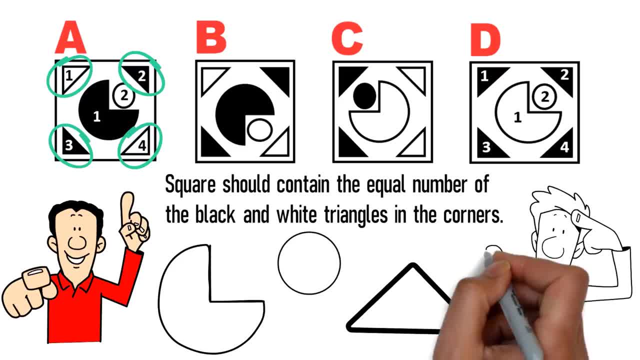 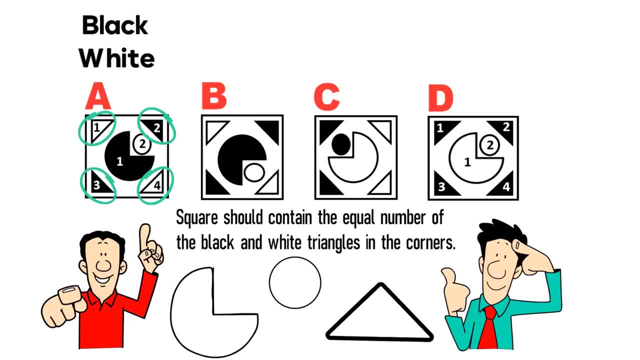 a pattern and their primary goal is to confuse you. if you look at the circles closely, you see that the large, small circle pattern doesn't exist. we have black- white, shape b- black- white, shape c- white- black and then shape d- white- white. based on this information about the circles, 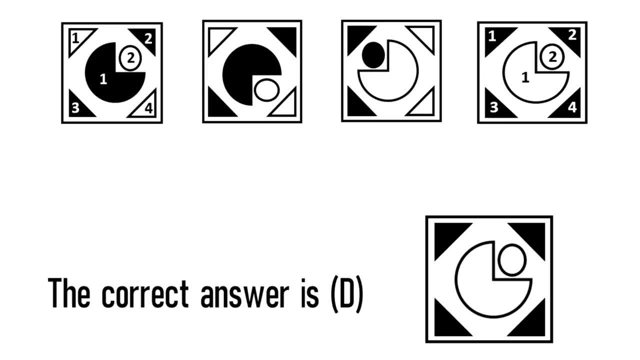 we should ignore them and focus on the triangles inside the squares. this is why the odd shape, the shape that doesn't belong to the group, is the one that does not have equal distributions of all colors in the corners. so the correct answer here is choice d. hopefully you've nailed this question. 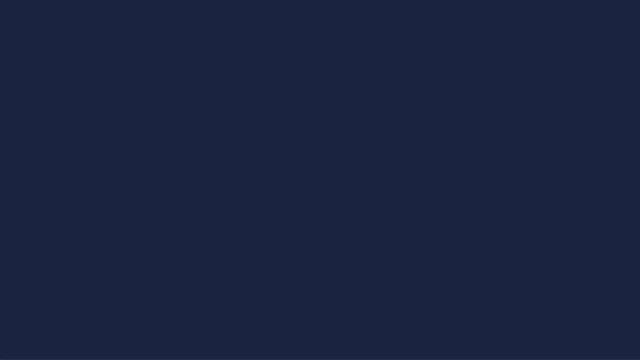 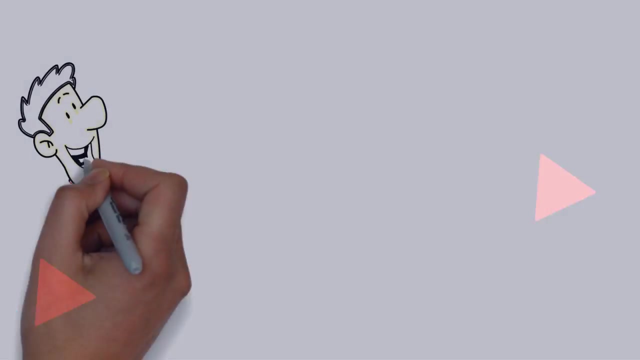 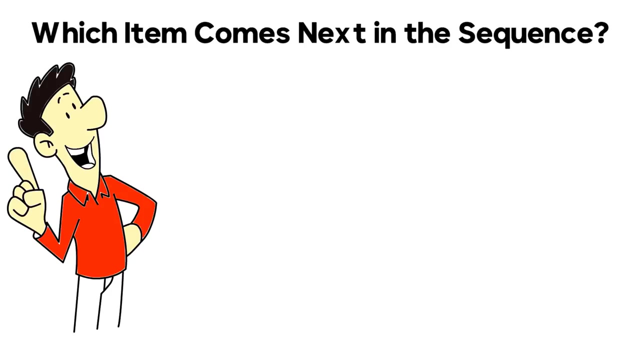 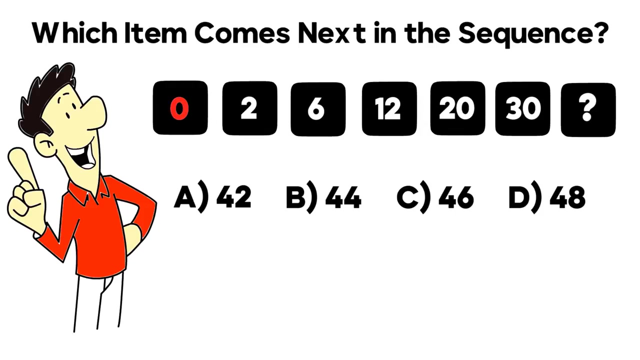 and now know how to answer similar problems on the test. very frequently on the test you might be asked to detect the pattern. in this question we're being asked which item comes next in the sequence and we're presented with the sequence of items. six items in the sequence are visible: zero, two. 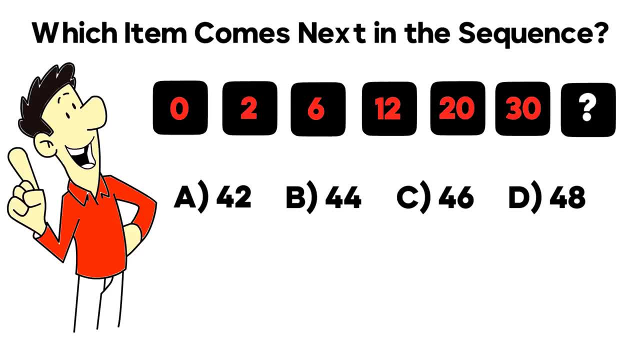 six, twelve, twenty and thirty, and the next item is missing and you're being asked to select one of the four following choices: choice a, 42, choice b, 44, choice c, 46 and choice d, 48. do you see the answer? it may or may not be obvious, depending upon your skills of detecting the path. 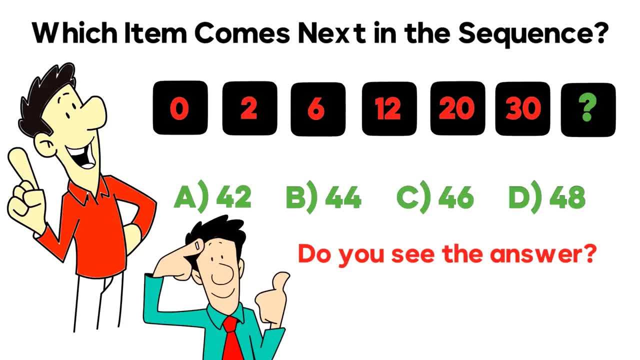 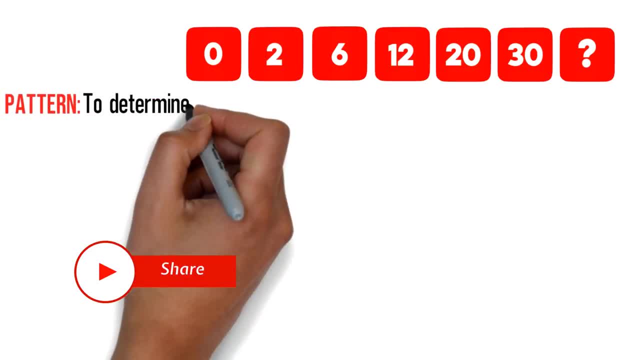 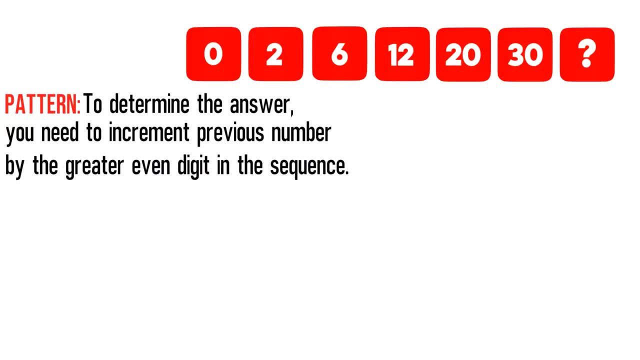 like it or not. we're gonna continue and i'll share with you the answer. as with any type of question, the key is to determine the pattern, to determine the answer. in this particular case, you need to increment previous number by the greater even digit. in the sequence, you can even come up with the formula and, in our case, the formula to determine the next. 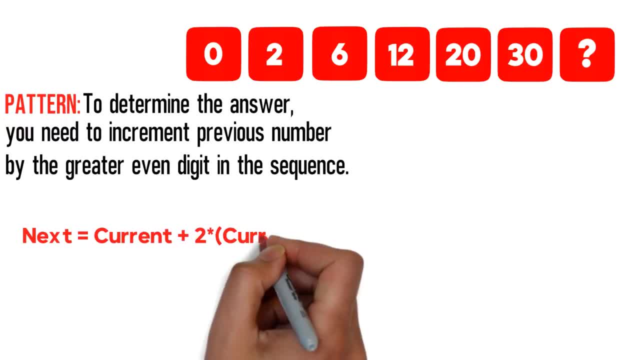 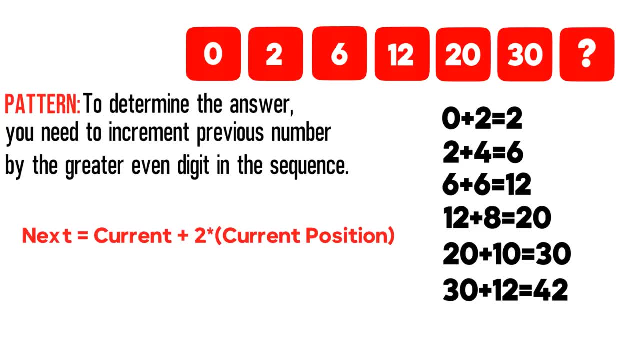 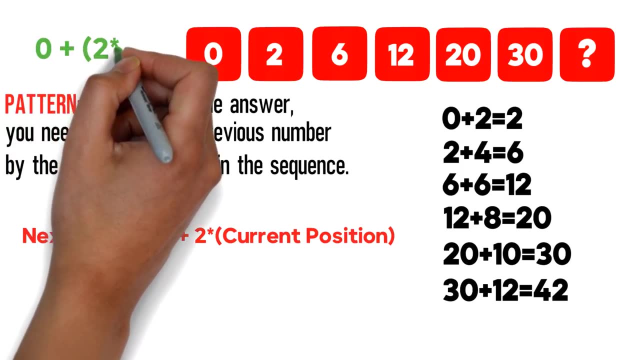 number would be current number plus 2 multiplied by current position. let's see how it works. for example, let's take the number 0. this is the first number in the sequence. to determine the next number in the sequence, we need to add previous number, which is 0. 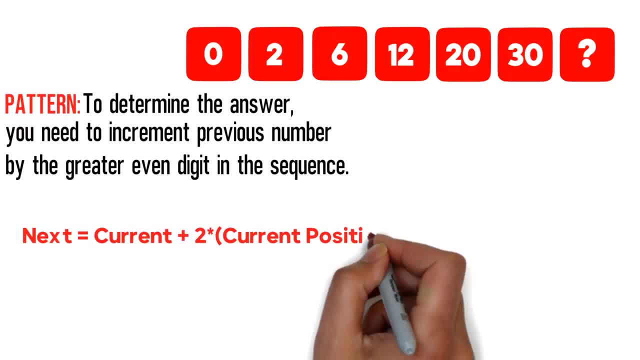 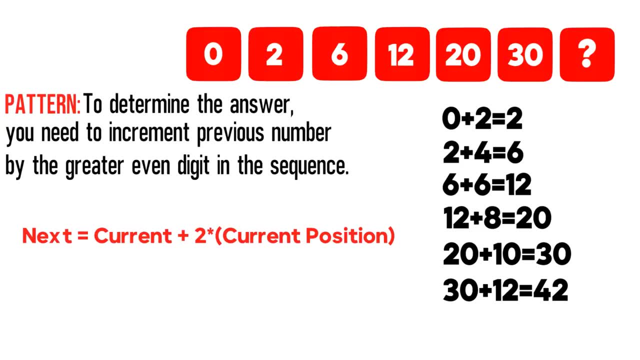 would be current number plus 2 multiplied by current position. Let's see how it works. For example, let's take the number 0.. This is the first number in the sequence. To determine the next number in the sequence, we need to add the previous number, which is 0,. 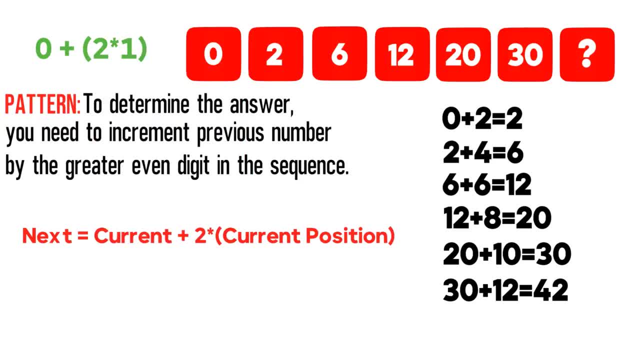 and then 2 multiplied by 1, because number 0 has the first position in the sequence, Instead of using the formula, you can also use the next even number and add it to the previous number. The even numbers are 2, 4. 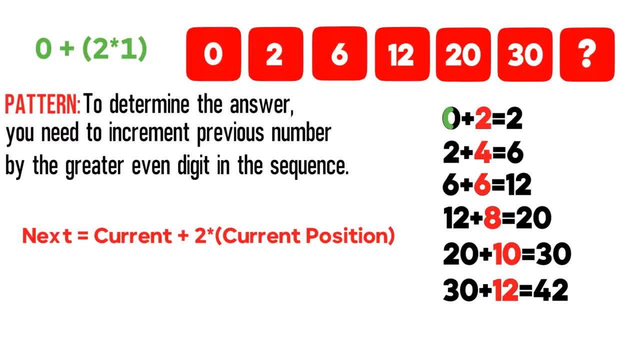 6 and you can increment them down the list, So you can add 2 to 0.. The next one would be 4.. 2 plus 4 equals 6.. The next number would be 6.. 6 plus 6 is 12.. 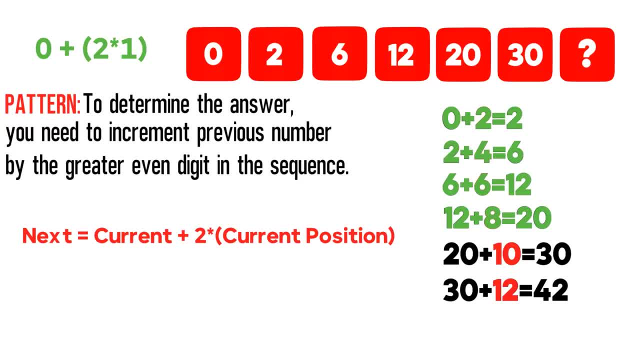 The next number would be 8.. And 12 plus 8 equals 20.. The number after that would be 10.. So 20 plus 10 would be 30. And the number after that would be 12.. And 30 plus 12 equals 42.. 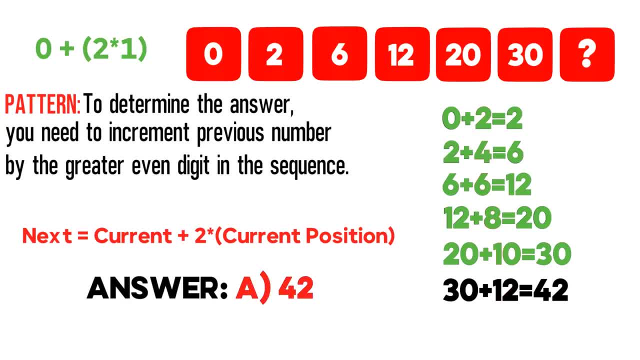 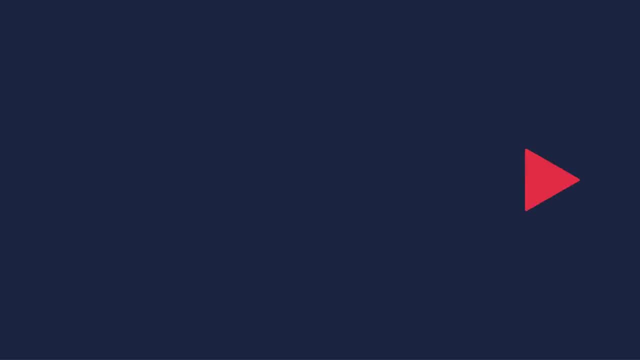 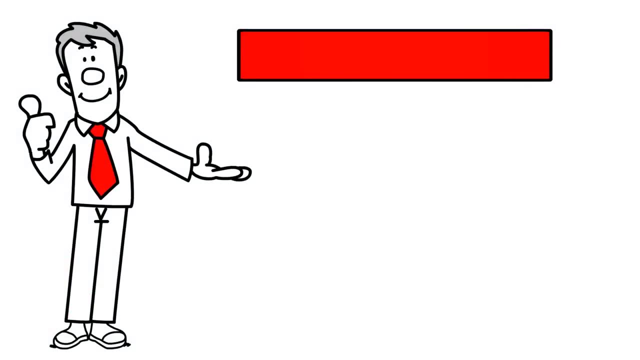 The correct choice here is choice A 42.. Hopefully you've nailed this question and now know how to answer similar problems on the test. I'm very excited to present you with simple but, at the same time, very tricky question which tests your math skills as well as attention to details. 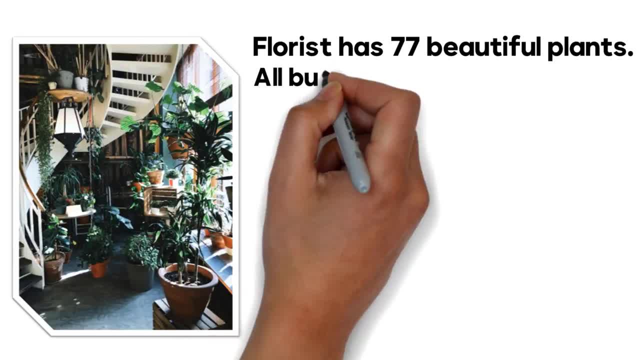 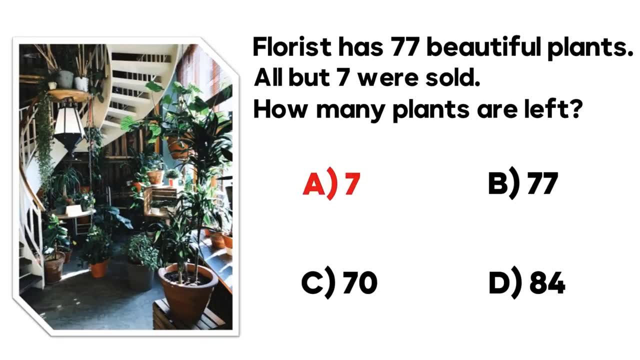 Florist has 77 beautiful plants. All but 7 were sold. How many plants are left? You have 4 different choices: Choice A: 7. Choice B: 77.. Choice C: 70.. And choice D: 84.. 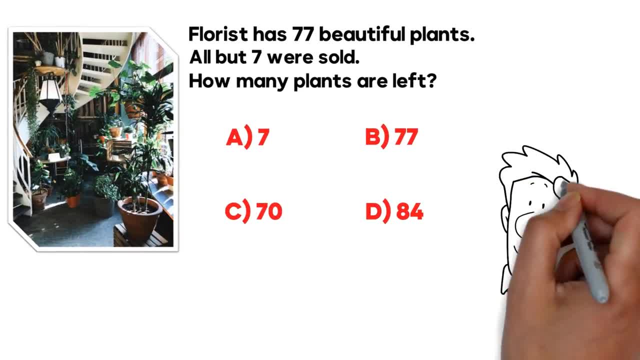 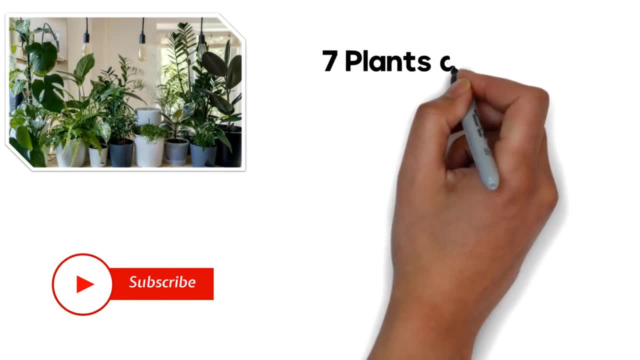 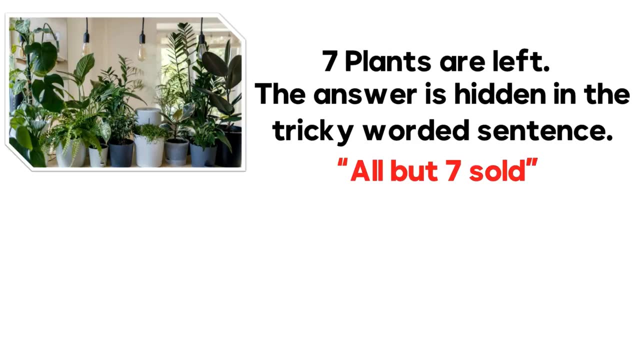 Do you think you know the answer? Let's continue to see how we can get to the correct solution together. The answer to this question is very simple: 7 plants are left. The answer is hidden in a tricky worded sentence. All but 7 sold. 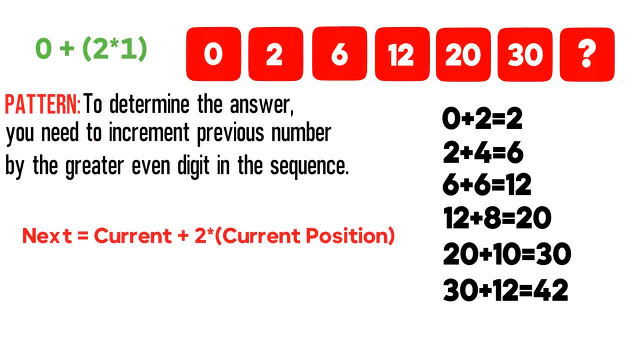 and then 2 multiplied by 1, because number 0 has the first position in the sequence. instead of using the formula, you can also use the next even number and add it to the previous number. the even numbers are 2, 4, 6, and you can increment them down the list. 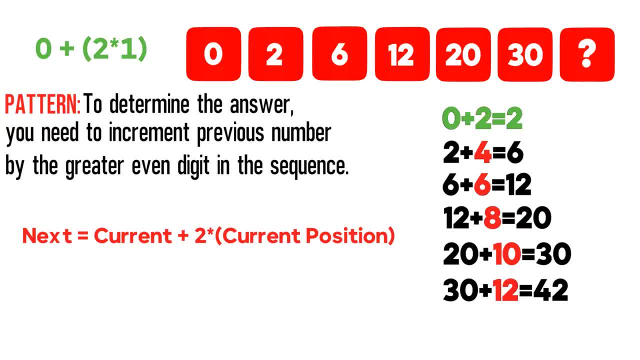 so you can add 2 to 0. the next one would be 4. 2 plus 4 equals 6. the next number would be 6. 6 plus 6 is 12. the next number would be 8, and 12 plus 8 equals 20. the number after that would be 10. 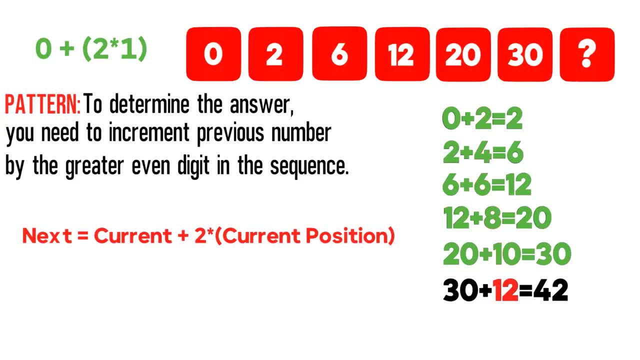 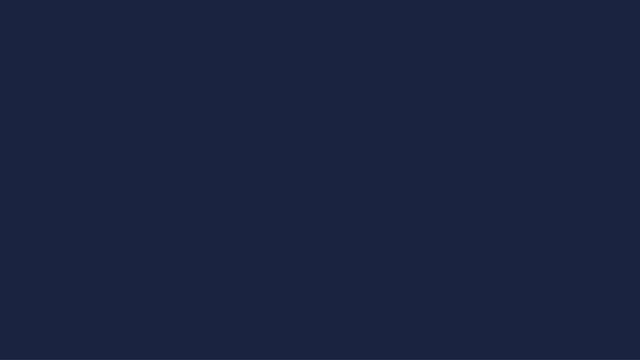 so 20 plus 10 would be 30 and the number after that would be 12. and 30 plus 12 equals 42. the correct choice here is choice a, 42. hopefully you've nailed this question and now know how to answer similar problems on the test. i am very excited to present you with simple but 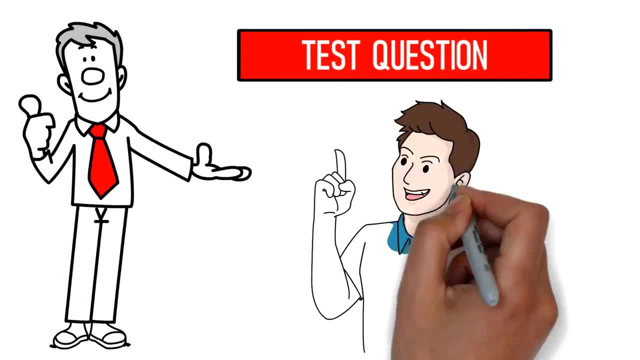 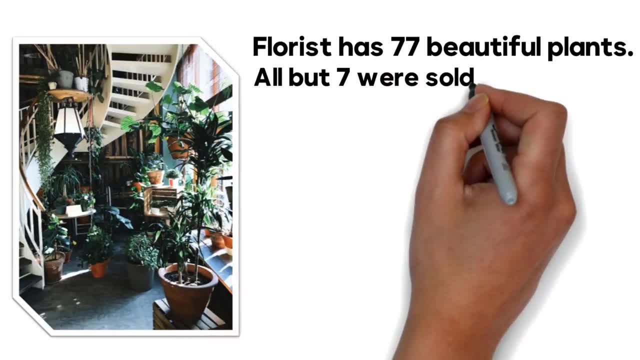 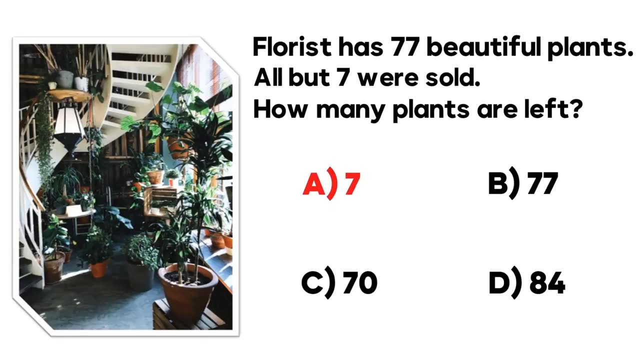 at the same time very tricky question which tests your math skills as well as attention to details. florist has 77 beautiful plants. all but seven were sold. how many plants are left? you have four different choices: choice a- 7, choice b- 77, choice c- 70 and choice d- 84.. do you think you know the answer? let's continue to see how we. 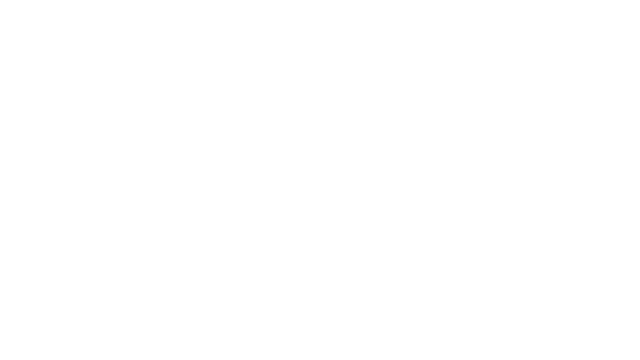 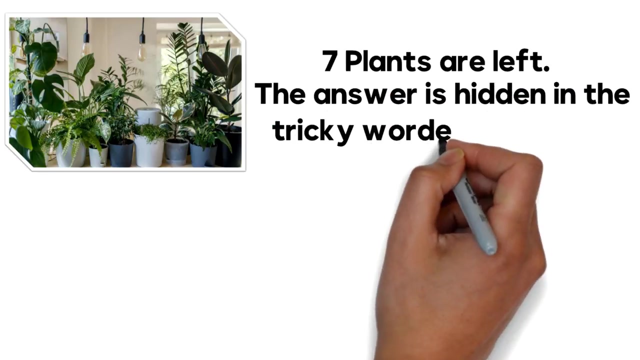 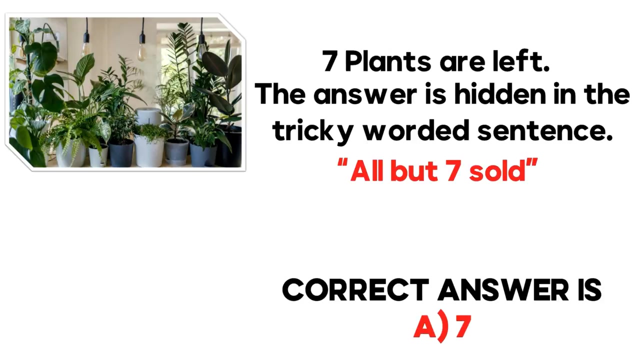 can get to the correct solution together. the answer to this question is very simple: seven plants are left. the answer is hidden in the tricky worded sentence: all but seven sold, so the correct answer here is choice a 7.. hopefully you've read this question correctly. 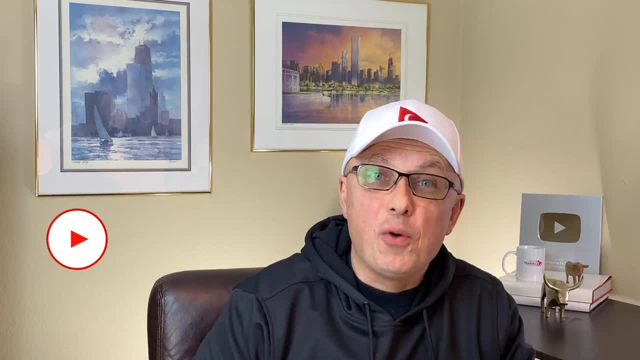 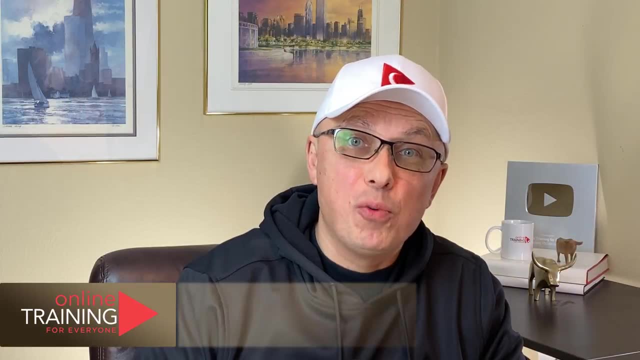 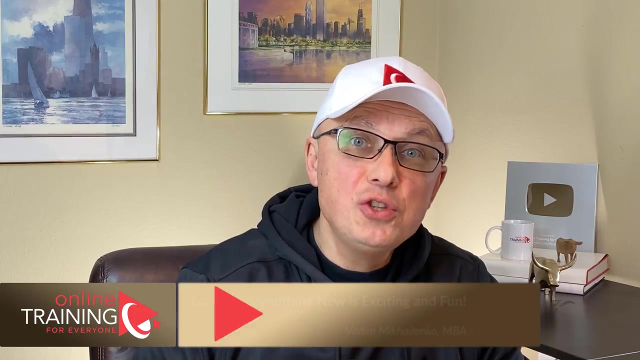 understood it very well and solved it on your own. thanks for watching. if you like the content, please give us a like and consider subscribing. thank you for your endorsement, support and patronage. please also check out additional resources in the description section of this video. i also encourage you to check resources page on our website, howtoanalyzedatanet. 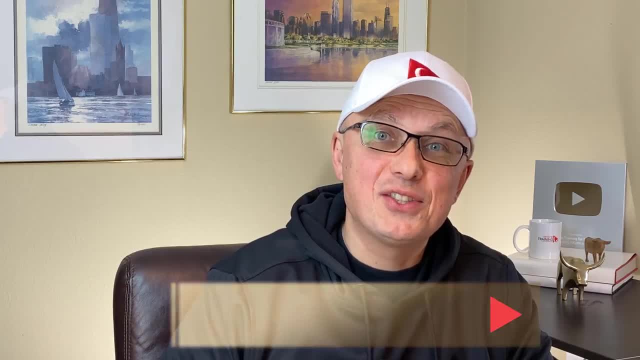 please leave your feedback, corrections or suggestions in the comment section of this video, and all the best on your journey. i'll see you in my next video. 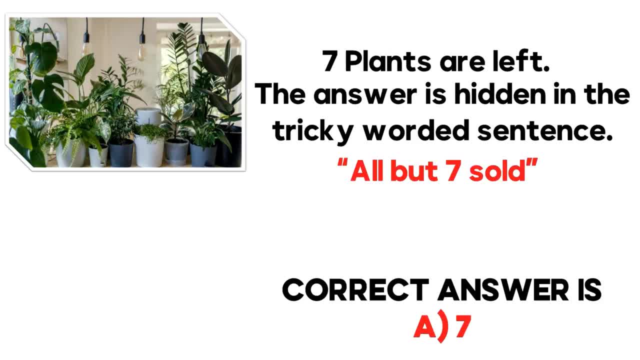 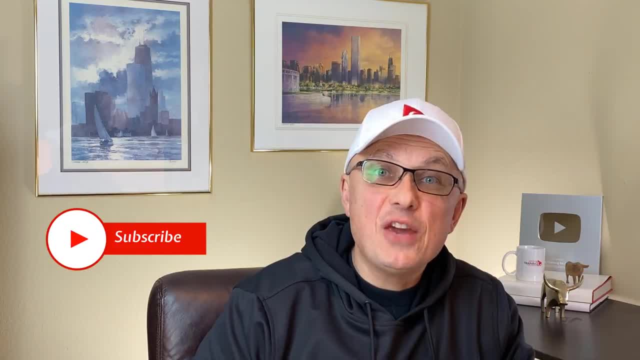 So the correct answer here is choice A 7.. Hopefully you've read this question correctly, understood it very well and solved it on your own. Thanks for watching. If you liked the content, please give us a like and consider subscribing.